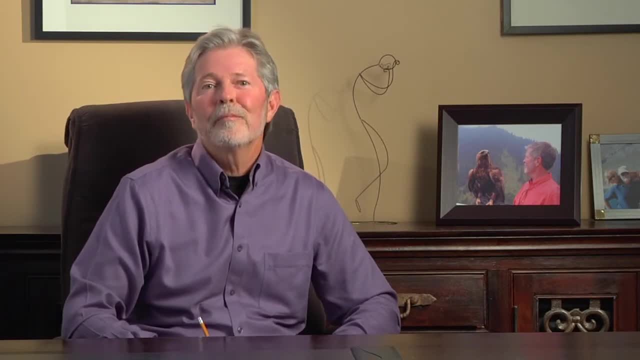 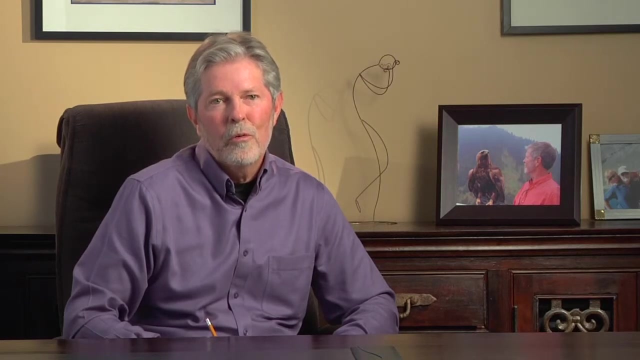 fearful, mad, irrational or just plain crazy. It is entirely my discretion as to whether I accept his price or simply close the door on him. Buying and selling is entirely at my discretion. Remember Ben Graham's words: the market does not drive your decisions, You make those decisions. 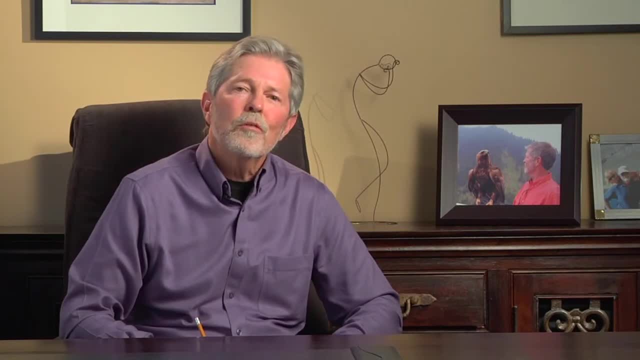 yourself. One of the ways to make those decisions is to attempt to do so with a mathematical model. These models assume rational behavior, and when Mr Market is rational, the models tend to work quite well. For example, a simple model might be what's called a stop-loss. 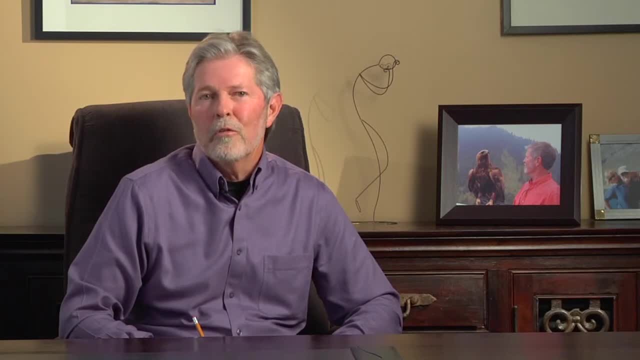 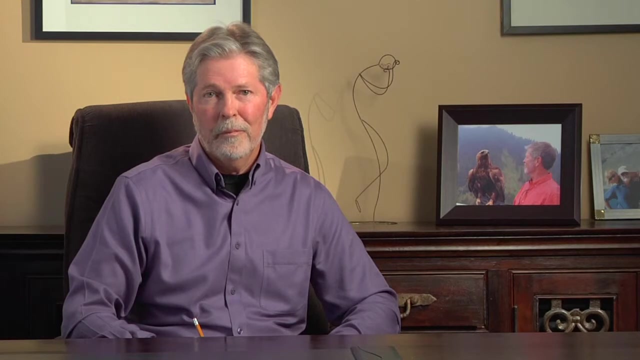 You might buy a security at $20 a share, willing to accept the loss of 10% of that capital If that stock goes down to $18 a share. your computer tells you that and you pull away. You sell it at $18.. You accept the fact that you've made a mistake. my bad. 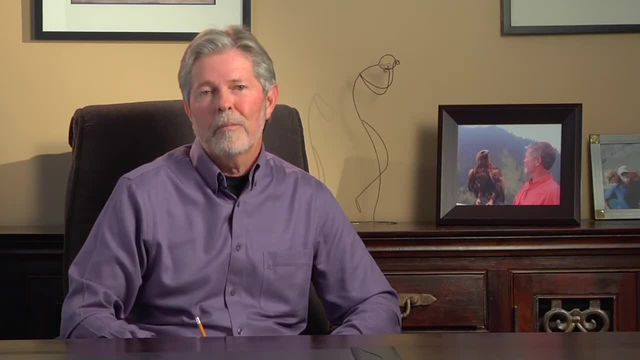 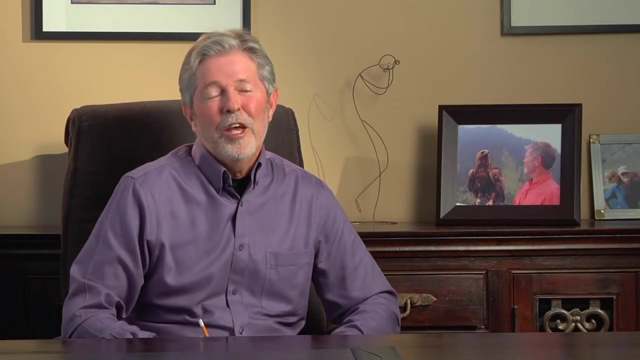 That's a stop-loss. It's a very simple mathematical model. More complex models may have to do with moving averages, Moving averages, Bollinger Bands and, even more complex approaches, econometrics. If you have millions of dollars, you can even buy a few dozen servers. put them next to. 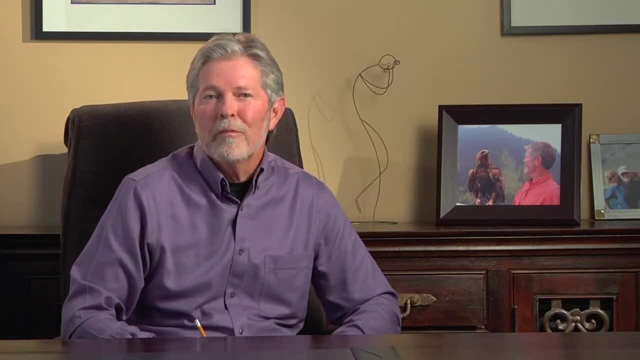 Wall Street and try to make money on the movement of hundreds or tenths of a cent in the price of a stock. These people are called high-speed traders. Their intent is simply to make money by manipulating the market. Technical analysis is the broad definition of mathematical models, As opposed to technical. 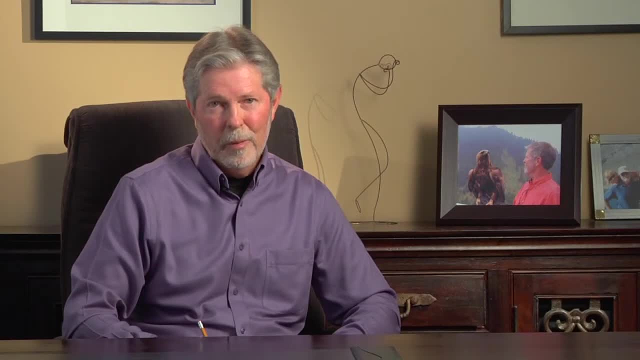 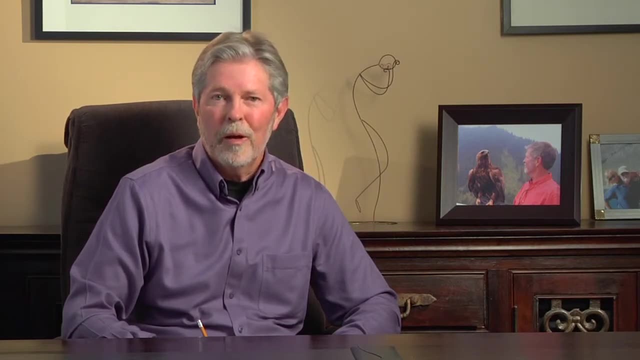 analysis. you have fundamentals. Fundamental analysis steps back from the marketplace, looks at the fundamentals of the product or service that a company may provide. looks at its financial statements, at its management team, at how it spends money and makes money, and makes decisions based upon more basic assumptions. 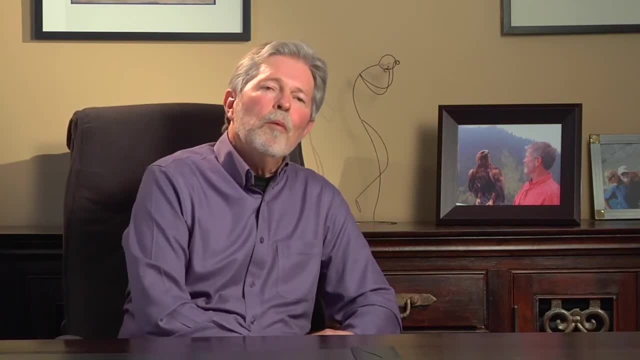 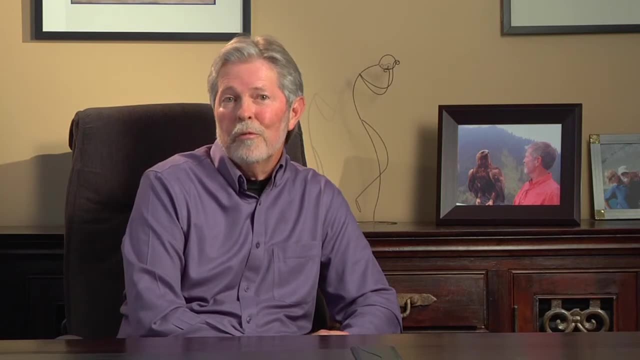 The fundamental analysis is the broad definition of mathematical models As opposed to technical analysis. you have the classical and the abstract. Remember when we were children, we played with models: Ship models or car models. Or little girls play with dolls. Those models were approximations of reality. The dolls,